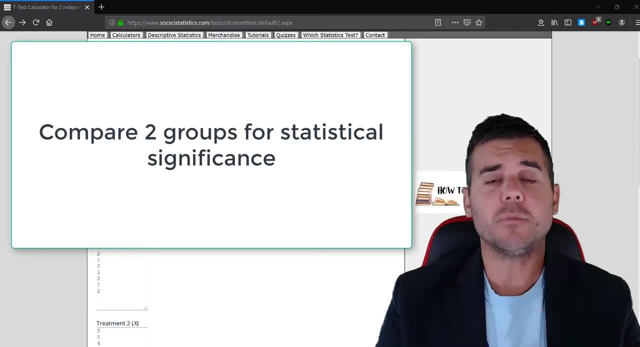 Now, if I have more than two groups, if I have multiple variables- and I'm looking at something else besides this comparison- you're going to do a completely different statistic, not a t-test. I'm showing you how to do a very basic comparison between two groups. 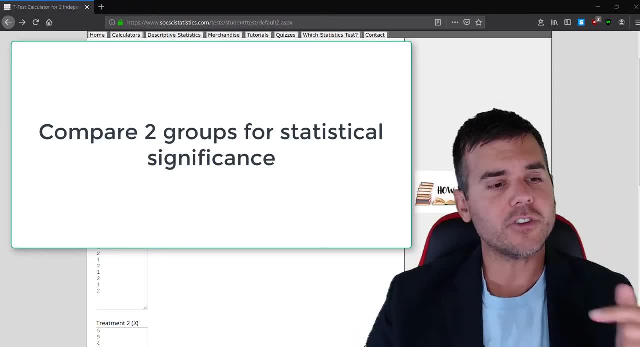 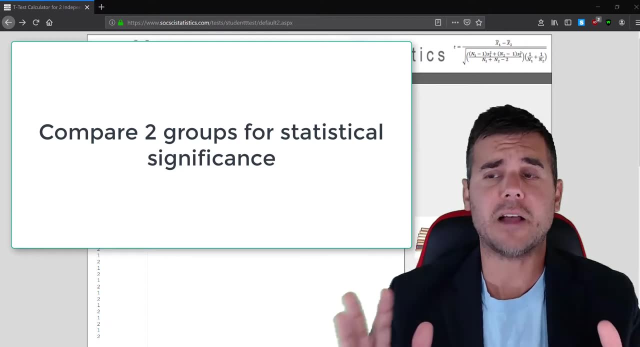 Okay, it's really easy to do. Let me show you how to do it. So let's look at the screen here and what I've done is I have entered in. I've just typed in Google t-test calculator. There's tons of them out there. So just search Google t-test calculator. You're going to find like: 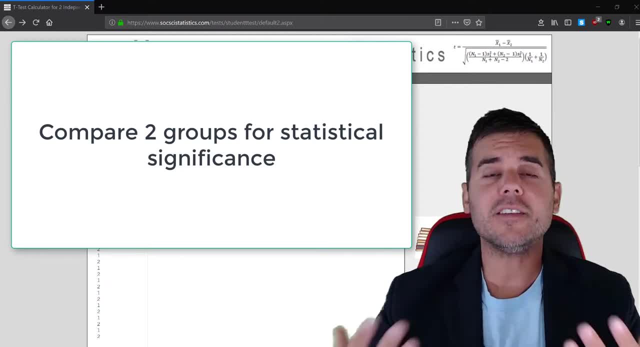 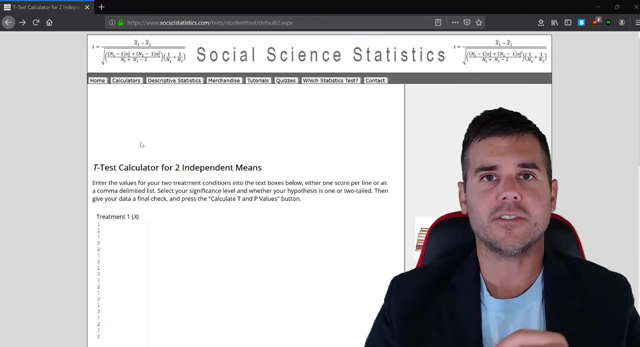 20 of them. They all do The same thing. All right, so let's imagine that I am comparing a class, Actually two classes. I want to compare the satisfaction between two classes. They could rate my scores between one and five. The first group: I just gave my class to normal class. At the end I said: give me a. 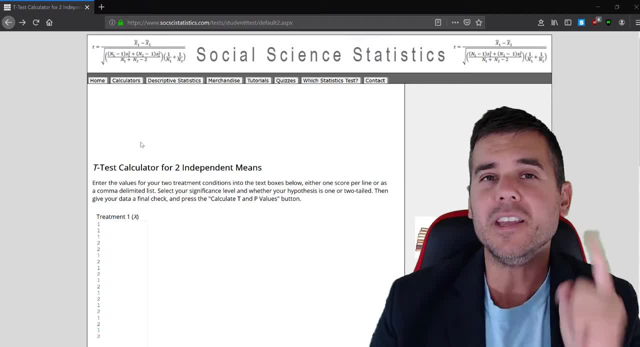 satisfaction report. The second group: I threw a pizza party at the end of the class. Then I gave them the test and told them the satisfaction and said: how do you rate my class? So, group one: no pizza party. I'm going to give them a satisfaction report. I'm going to give them a satisfaction report. 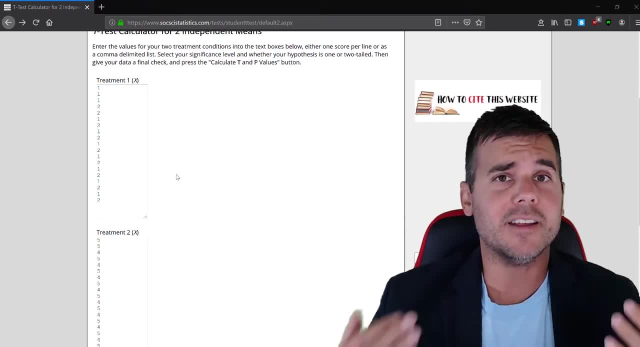 The first thing I like to do is just eyeball my data and see what does my data look like, Like without me running any stats whatsoever. what do I think I've got here? Okay, so ones and lots of twos. So that means it didn't sound like my students were that satisfied. They didn't like 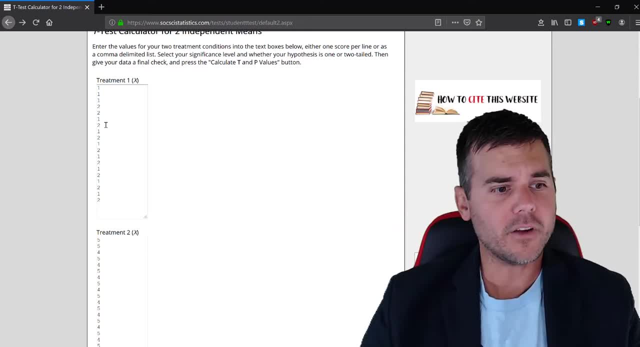 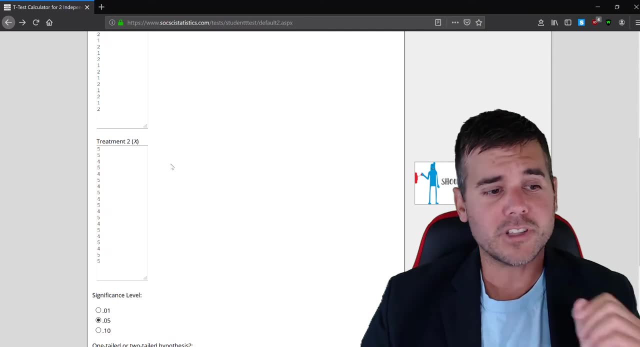 my class. How can I improve it? Okay, so class two: I threw a pizza party. Let's look at the satisfaction scores. We're just eyeballing this data. I see lots of fives and fours, which was the highest Way to go. I'm an awesome teacher, Or it was really good. 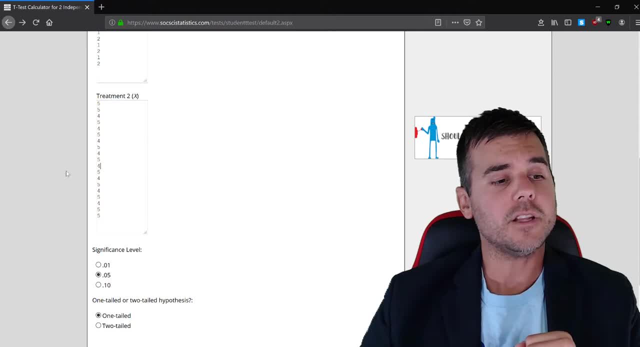 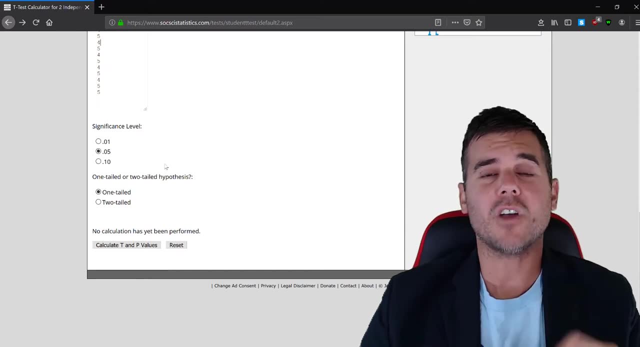 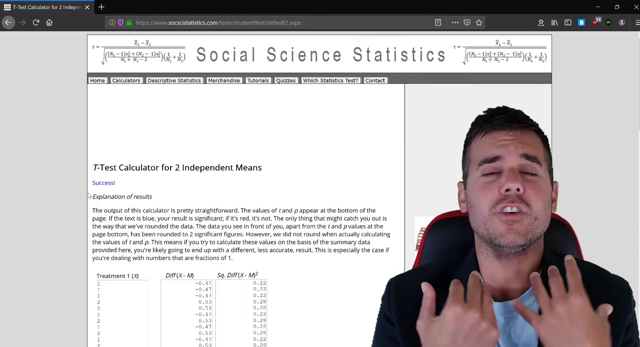 pizza. All right, so what I'm going to do, I'm not even going to touch anything here, So I'm just going to keep my significance level at 0.5.. That's the most common. I'm going to calculate my results. Okay, so when I calculate my results, they're going to show you tons of data. 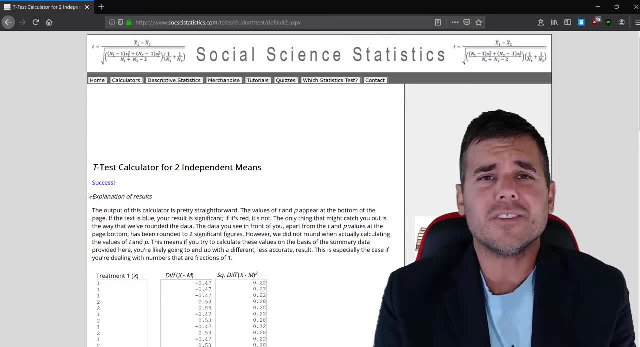 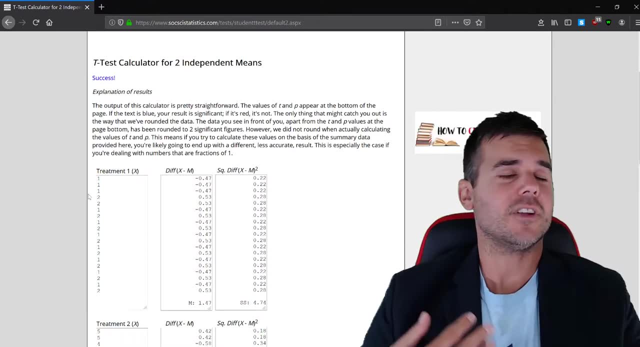 But you know you're not here for all this. You just want to see: is there a difference? and what was the difference? right, That's what most of us want to see. Okay, so they're going to give us a lot of different kinds. 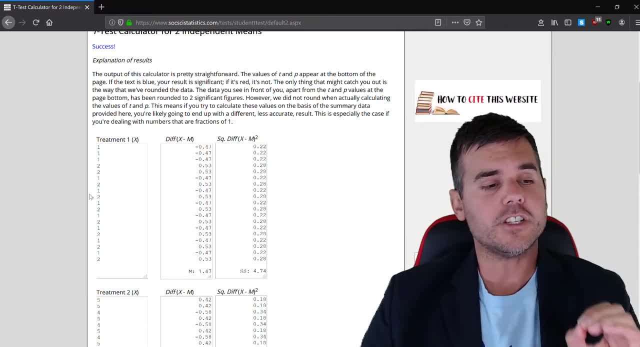 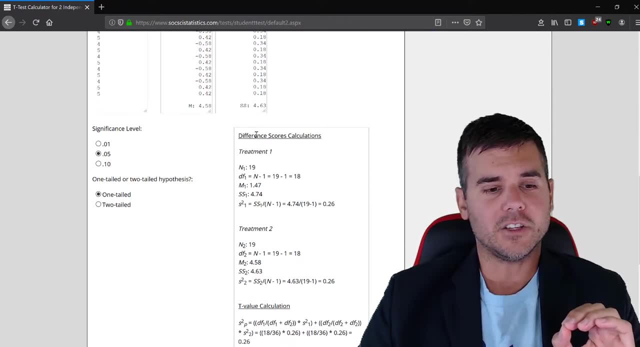 of data here, which is really good in some regards, But I'm going to show you just some of the key things that you want to look out for, All right, so the first things I want to look for is: I'm going to go over here and look at my data. You can see it here on the left. All right, first thing: 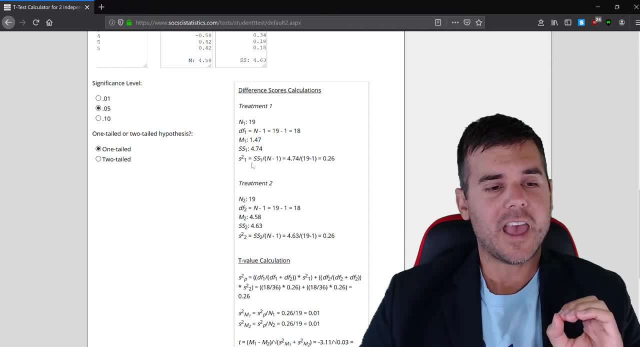 I want to look at are my means of each group. I see M1.. This is my mean. So the mean of group one was 1.47.. The mean of group two was 4.5. 8. So again, eyeballing those two means that's a big difference between the lowest and highest. 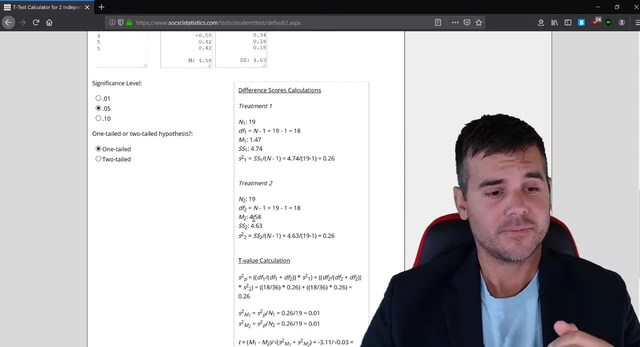 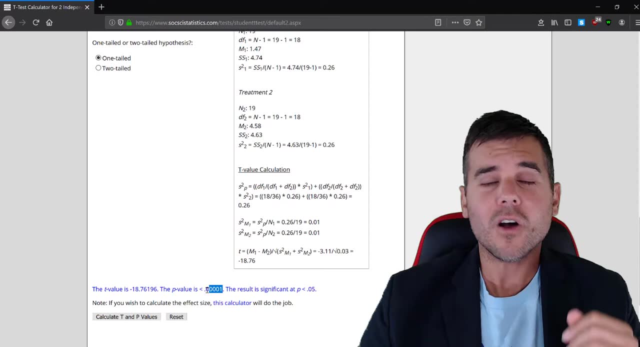 So it seems like there was a significant difference. Let's scroll down even further. Okay, the p value was point 00001.. The result is significant. p is less than point 05.. So what we're seeing is that I had a significant difference. Now, when I say something I'm not, 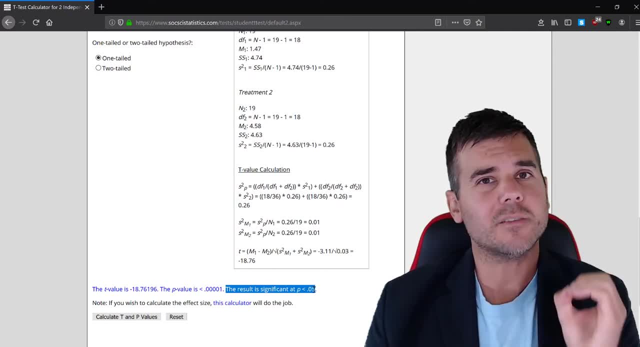 saying significant, I'm not proving anything. Statistics doesn't prove. So I'm never sending out to prove something. What I'm doing is I'm saying here: hey, I'm looking at this data, I'm eyeballing it. It looks like there's a significant difference here. When I run it. 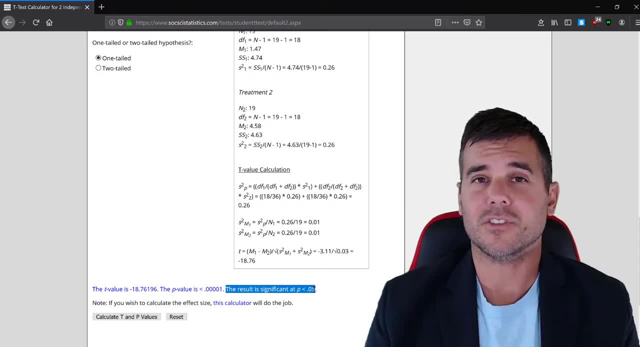 through a t-test. it's also telling me there's a significant difference. So it seems like this is I'm making a good case. Basically, what you're doing with stats is you're building a case to try to conclude something I'm not proving. I'm trying to draw a conclusion, So it looks like I'm. 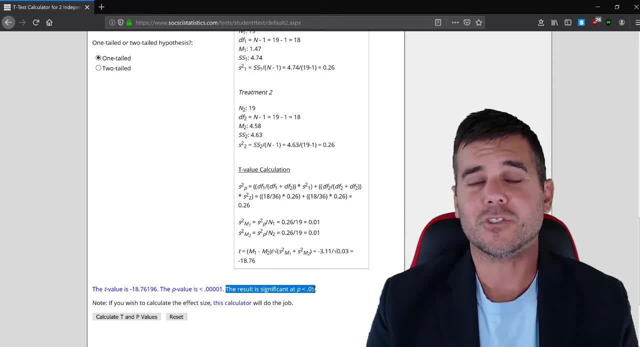 a really strong case that there's a difference. when you eyeball the data, There's a reason why I think there's a difference, which was the pizza party, And my statistics are now showing a significant difference. All those three pieces together helped me conclude that there was a. 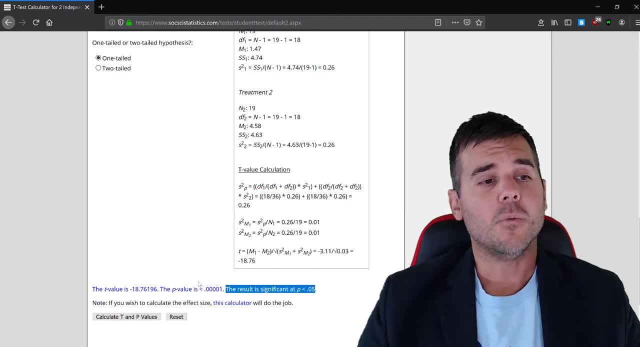 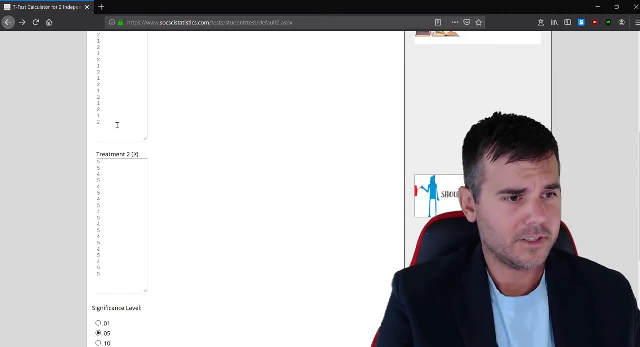 significant difference between these two classes. Now, one of the things I want to show you is, let's say, I mess up one of these data fields, All right, so I've just entered like 5 million into one of the data fields by accident.